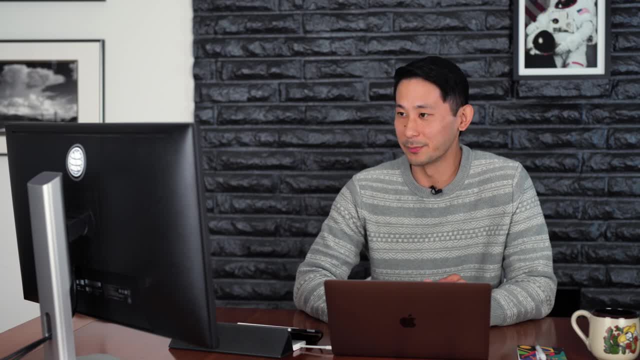 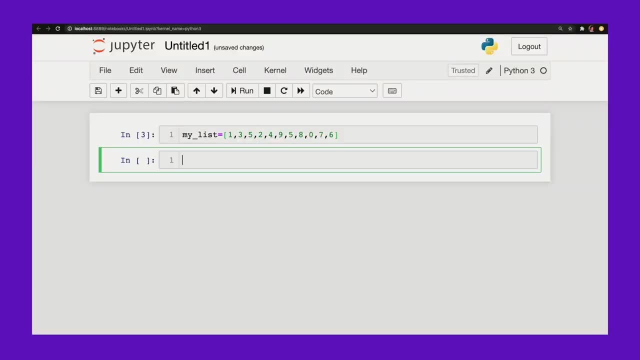 this list. How a classical computer would approach this problem would be to check each element of the list here and just see if that number is equal to my winner. And we can model this using what's called an oracle, And all this means is that we have a blackbox. 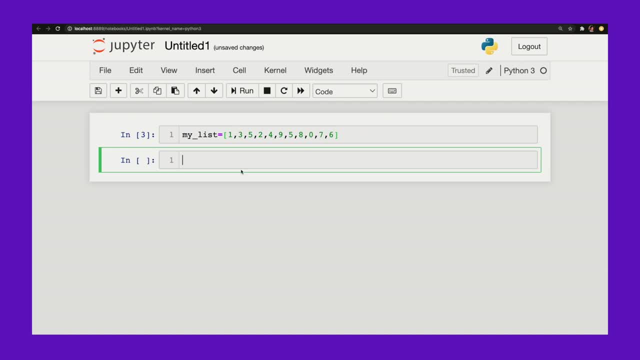 at our disposal and we can call it and ask it: is this number the winner, yes or no? so let me just define my oracle, my input and the with the oracle knows that my winner is the number seven and it'll just tell me, if i give it an element of the list, if that element is the winner. so if my input is, 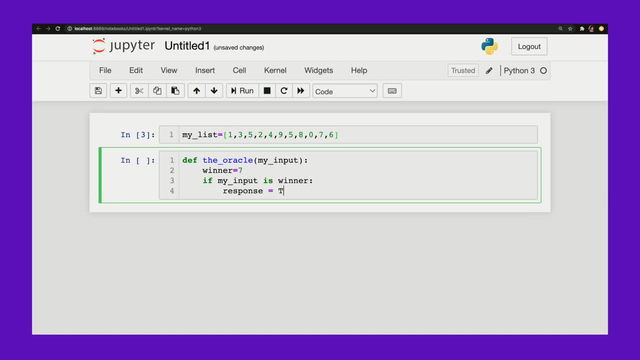 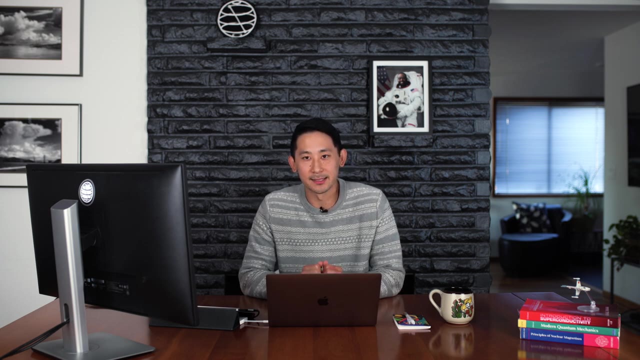 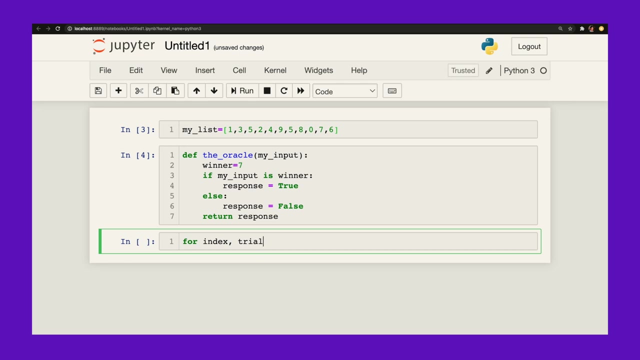 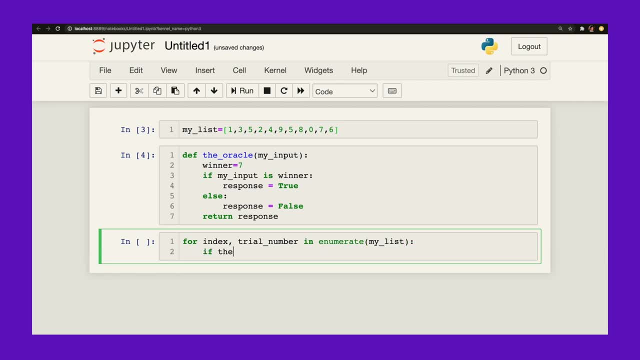 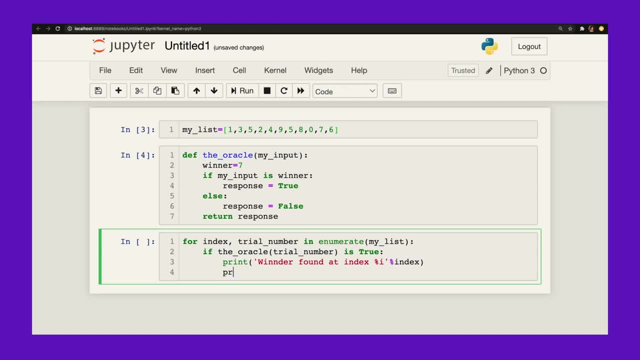 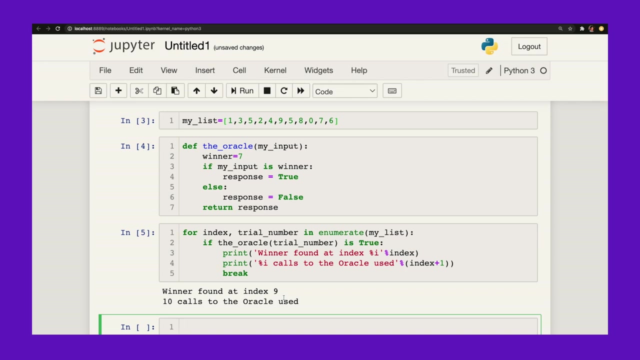 index and also also, oops, also tell me how many times i had to call the oracle and tailga and a complicator to and break okay. so what this is telling me is i had the oracle 10 times and the winner was found at index 9. 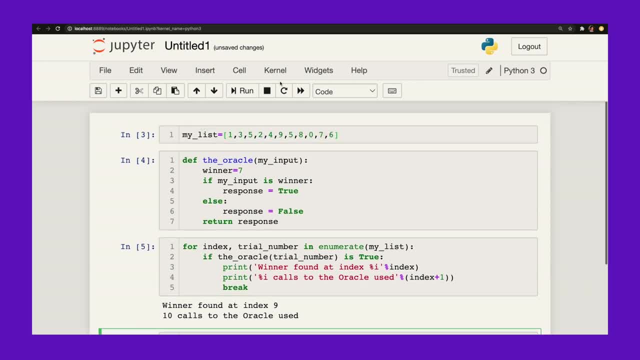 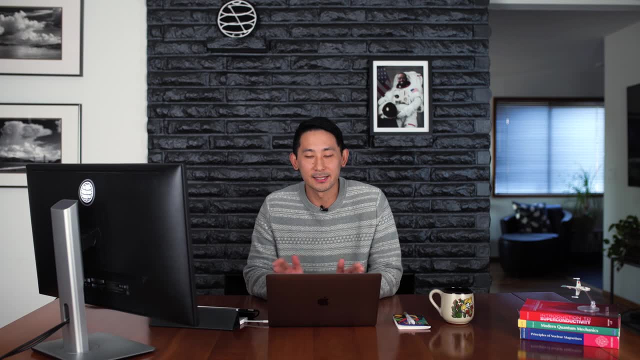 of my list list and we can just quickly verify that yep, seven is the ninth index of my list. so we use ten calls to the Oracle. so we see, for this list it took us ten calls to the Oracle. but we could also imagine a situation where I get lucky and my 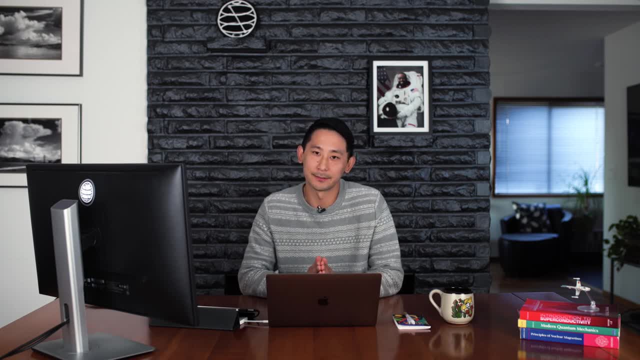 element is at the front of the list, so we would use fewer calls to the Oracle. so on average, the complexity of this problem requires us to call the Oracle n over two times on average. in the worst case I would have to call the Oracle n times if my element was at the very end of the list. so we say that the 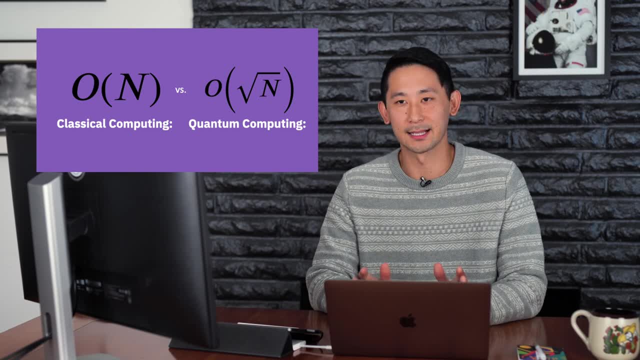 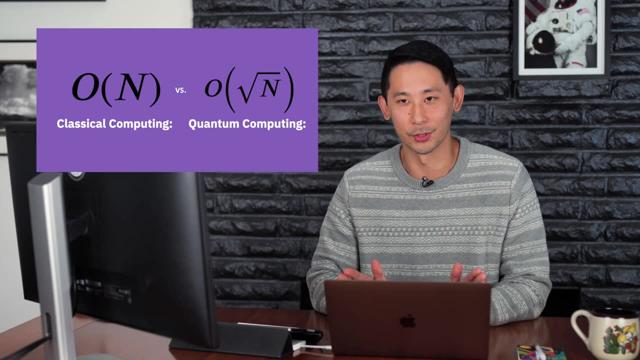 complexity of this problem scales as order n in the classical case. now the amazing thing about a quantum computer is that we can get away with only square root n calls to the Oracle by using Grover's algorithm. so let's get into how this algorithm works, the Oracle in the quantum case. I'm going to just model as: 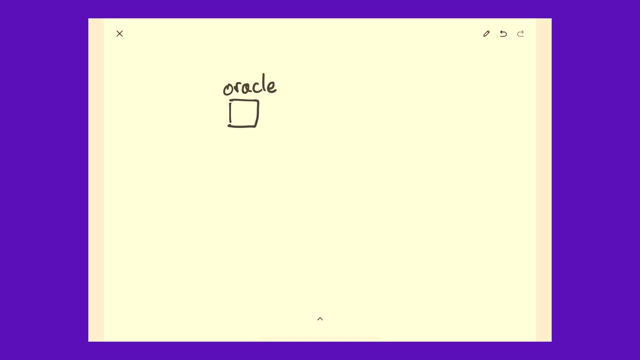 this black box Oracle and it's gonna be a function that will flip the sign of the input if the input is the winner. so we can encode our inputs as the basis state for the input and then we can use the input to encode the input as the. 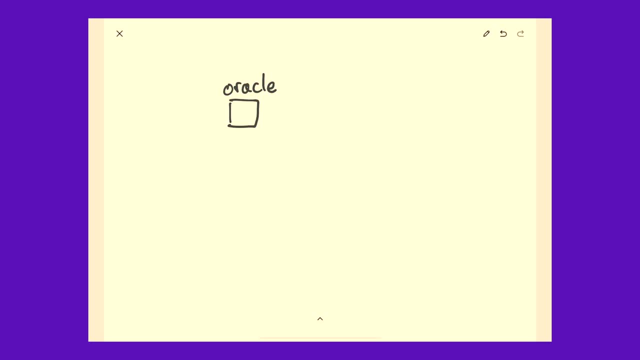 of a quantum computer. so remember, for two qubits we can represent four input states: 0, 0, 0, 1, 1, 0 and 1, 1. and let's suppose that our winner is the state 1, 1. so if we feed our state 1, 1 into our Oracle, where we get back is minus 1, 1 and 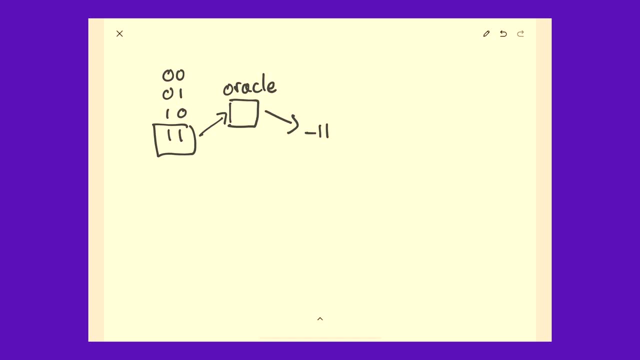 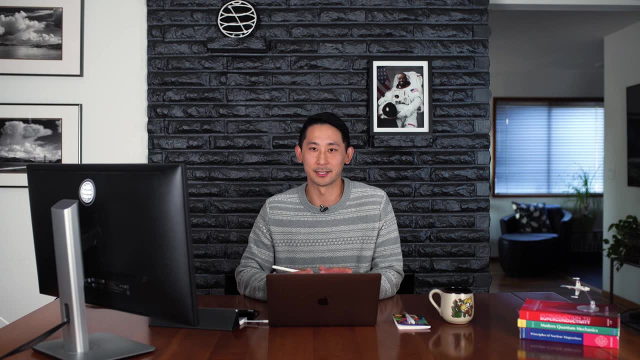 this is the way our Oracle is gonna work. it's gonna flip the sign of the input if the input is the winner, and the way we can change these states is through a unitary matrix which we can use to change the state of a quantum computer, which we can encode into a quantum circuit. so we want a circuit that flips. 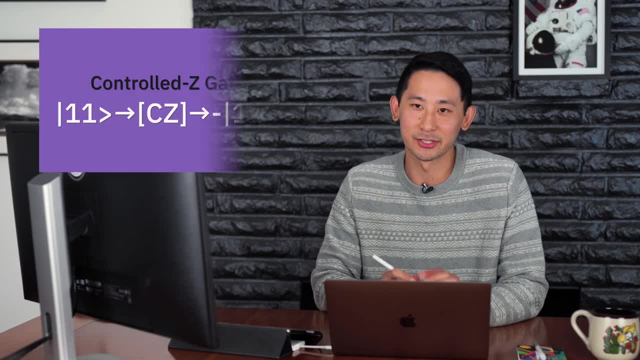 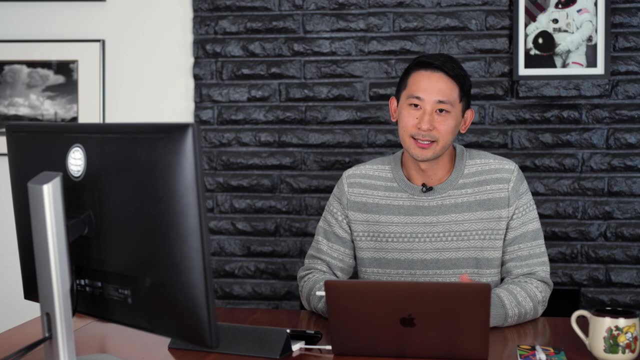 the sign of the 1- 1 state and, conveniently, we have a gate that does just that: the controlled Z gate. in addition, we'll need one more ingredient in order to do what's called amplitude amplification, and that ingredient is called the reflection operator. the combination of these two operators is: 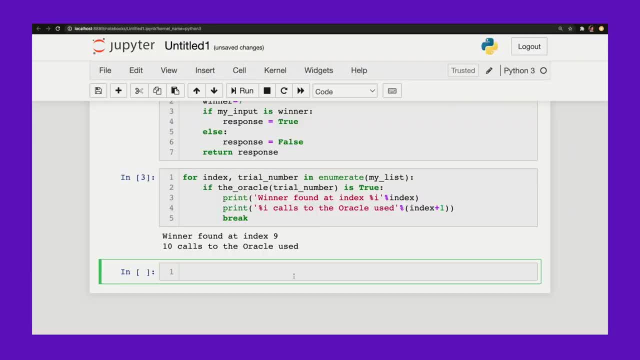 known as Grover's diffusion operator. let's see what this looks like in kiskit now. so from kiskit I will import everything. import mat plot, lib Unamphi as plot, so I can do my plotting, and I'll import numpy as NP, just so I can. 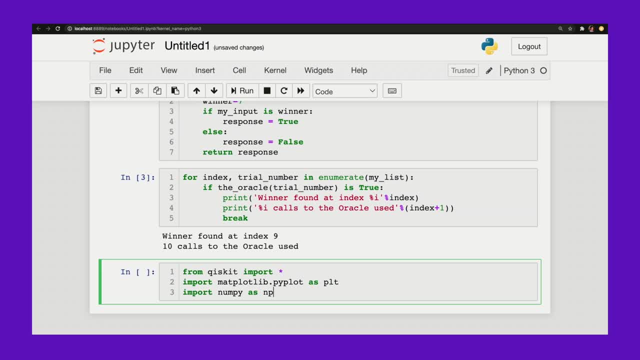 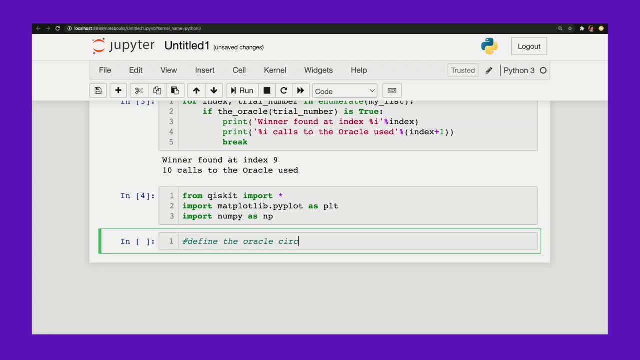 do some array stuff. okay, all right. so let me now define the Oracle circuit, so the Oracleiąg quantum circuit with two qubits. I'm just gonna deal with two qubits for now. i'm going to call this the oracle and, like i said before, there's a convenient gate that 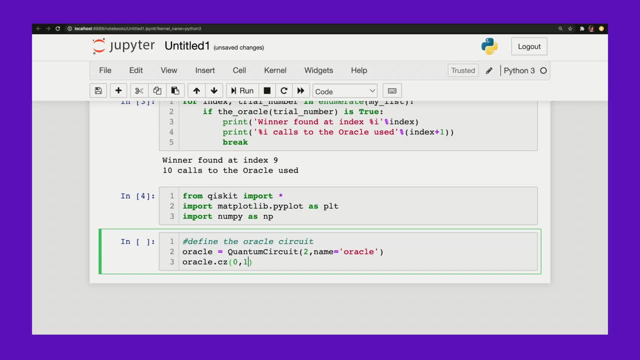 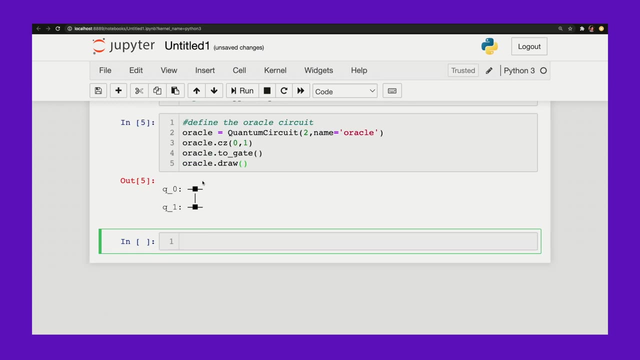 flips the sign of our winning state with the controlled z gate, and i'm going to make the oracle into its own gate. okay, let's see what this looks like: oracledraw. okay, that's my cz gate, which acts as my oracle. let's quickly check now that our oracle is doing what i want it to do. 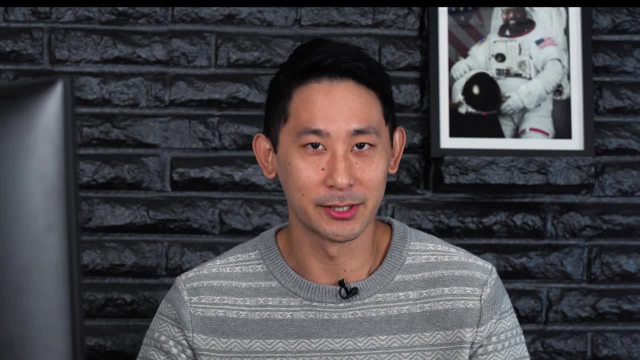 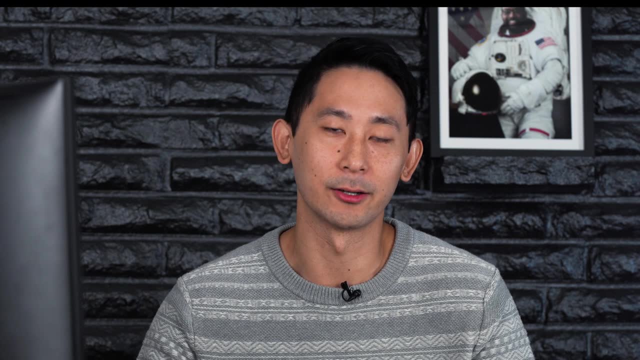 so i can check this by preparing a superposition state of all of my qubits, by applying a hadamard gate on each one of them, and this way i can query each one of the input states simultaneously to the oracle. i'll call the state s for superposition. 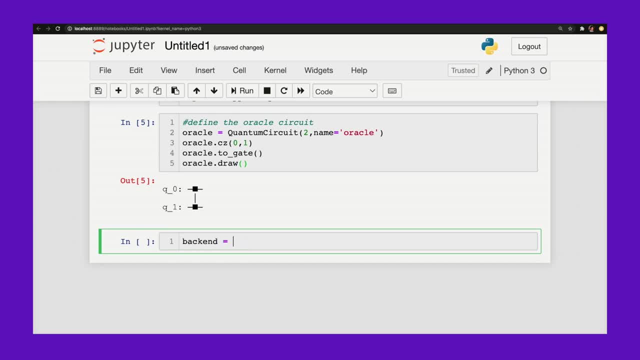 all right. so to check that the oracle is doing the right thing, i'm just going to call the simulator backend the state vector simulator. okay, i'm gonna define my grover circuit, quantum circuit, two qubits, two classical registers, grover circ, and i'm gonna add hadamard gates on both of my qubits. 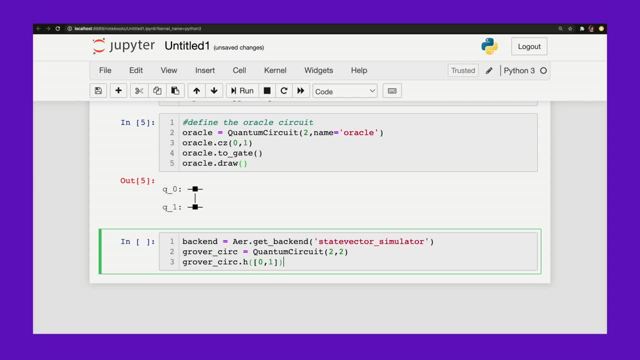 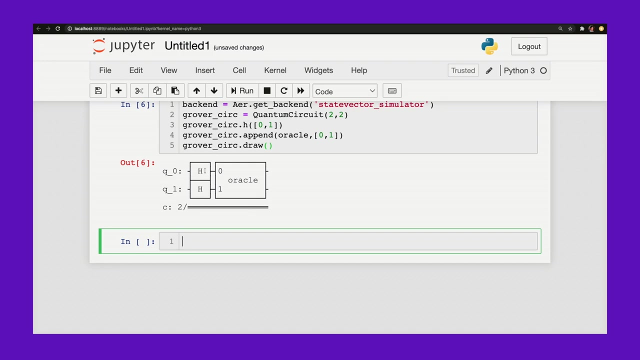 zero and one. this prepares my superposition state s, and then i'm going to add on my oracle so i can query each one of my states at the same time. okay, and let's once again draw this, so I know what it looks like. okay, good, so I am applying a Hadamard on each one of my input qubits. 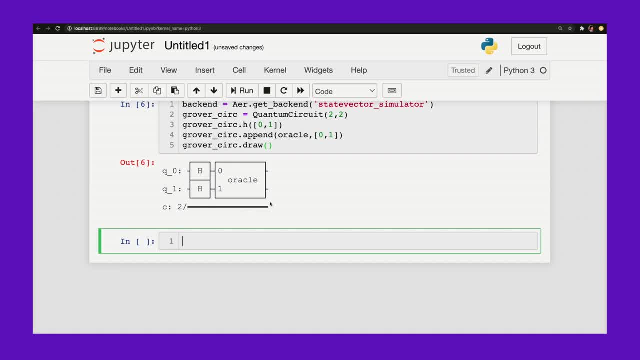 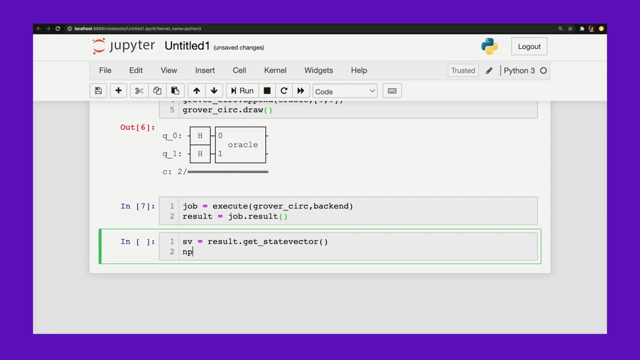 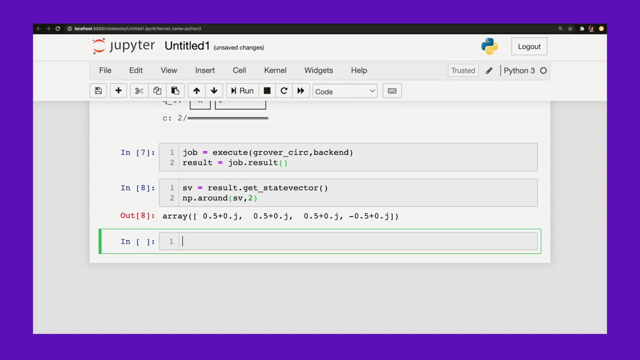 this prepares all four superposition states and then I feed them into my Oracle. so let's execute this job on the simulator. get back the result, okay, and let's get back the state vector, result dot. get state vector and I'm just gonna round these numbers off, okay, good, so we've prepared the 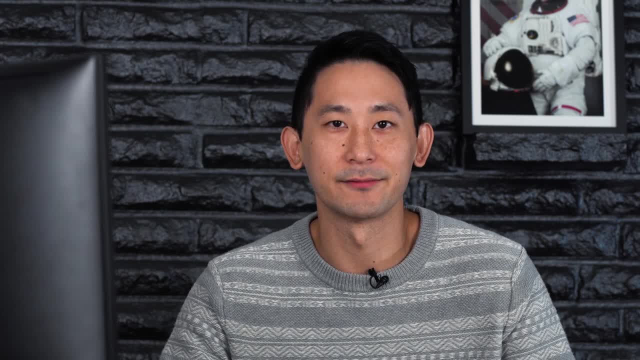 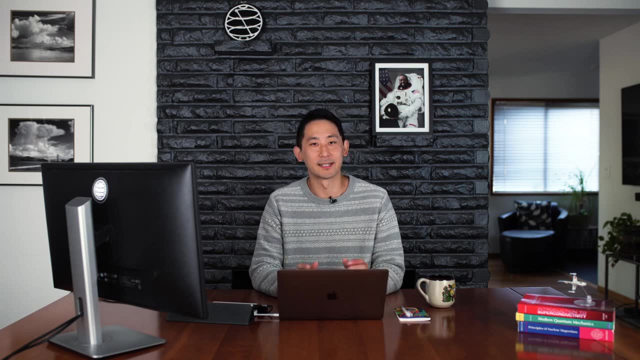 superposition state and we get back the same state, but with a 1-1 state flipped. so our job is done right, not so fast. in quantum mechanics we have to square the state vector. in order to get back the probabilities of measuring that state more precisely, we have to multiply each element of the state vector by its 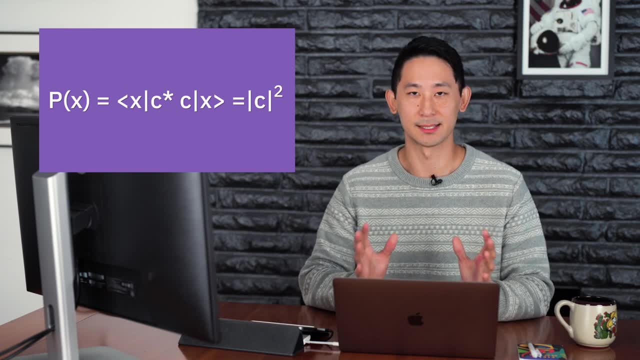 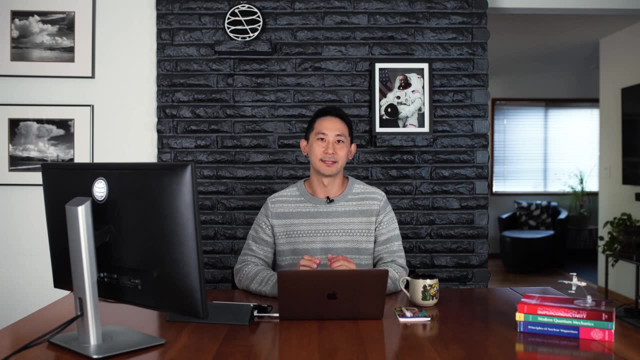 Hermitian conjugate in order to get the state vector to get back the probability of measuring that basis state. so the minus sign in the state vector will never actually show up in any measurement that we do. at this point we need one more ingredient to tie all of this together. 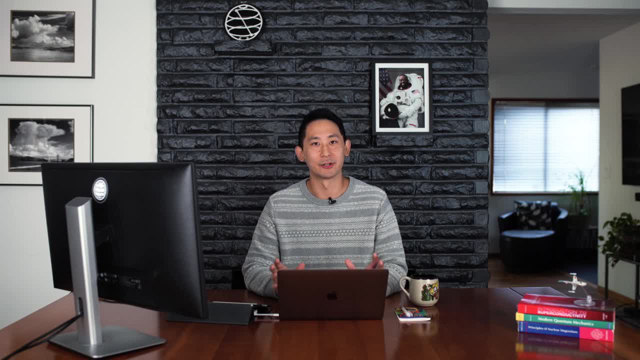 the reflection operator. with the Oracle and the reflection operators we can do something called amplitude amplification. with amplitude amplification we can amplify the probabilities of the winning state, W, and we can reduce the probabilities of all the non winning states. let's talk about how the amplitude amplification works now. there's actually a 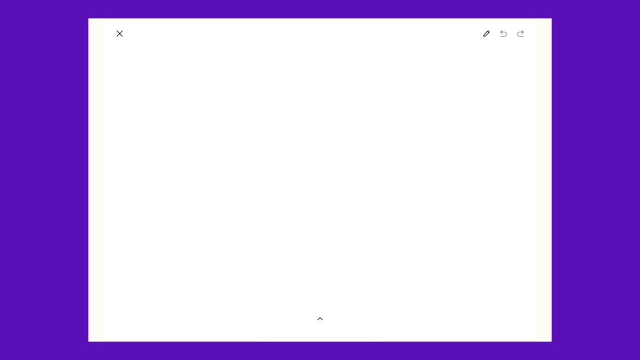 really nice geometrical interpretation of how this works. so let's think about our winning state W and our superposition state S, and our winning state is represented as this vector: 0, 0, 0, 1, and this is equal to the 1: 1 state. 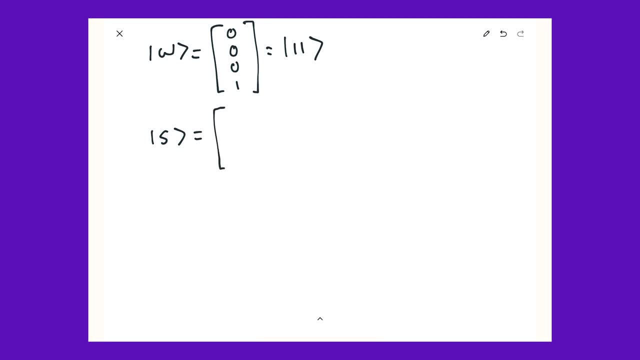 the superposition state is represented as this vector: 1, 1, 1, 1, where each one of our input states is equally likely and normalized by 1 half. so we can think about these two states as vectors in space which are almost orthogonal, or almost at a right angle, but not quite, and we can come up with a new state. 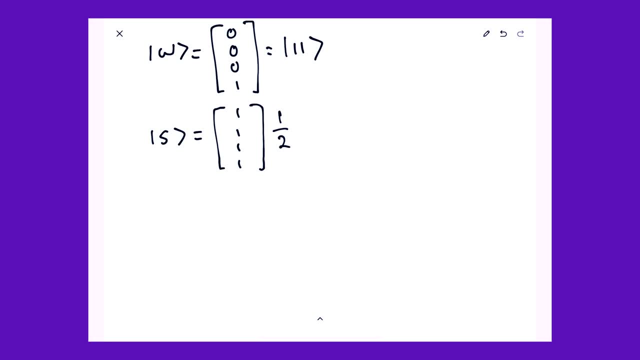 within the span of W and S, which we'll call S prime, which is actually orthogonal to W. so this will be defined as 1 1, 1, 0 and with a normalization factor you can actually check that W and S prime are orthogonal to each other. so you'll notice that S prime is just the S state. 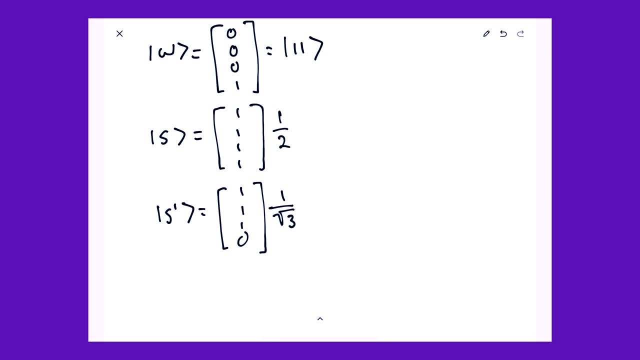 with the W component removed from it. so let's draw what these vectors would look like in space. here I'm drawing my W vector. here's my winning state and, like I said before, the S state is almost orthogonal to it. And we've constructed our S prime state so that it is orthogonal to W. So this is the 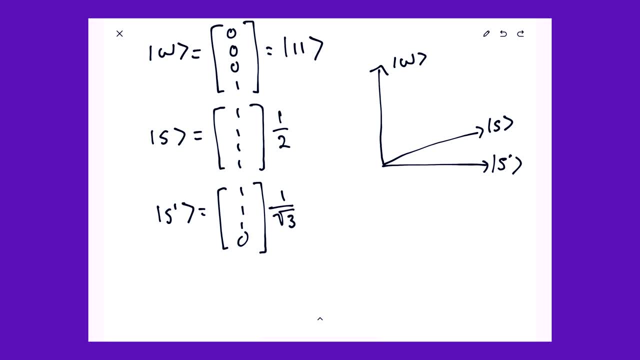 right angle here. So now when we apply the oracle operator to S, so our S goes into our oracle, the oracle flips the sign of the winning state. So what comes out is this vector, one, one, one minus one, and our normalization factor. So now when we apply the oracle operator, 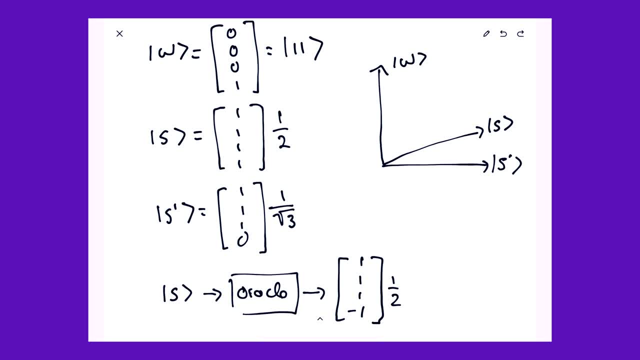 to S. we flip the sign of the winning component. So geometrically, this means that we reflect our original S about S prime. So we get a new vector that looks like this: So our S has been reflected around S prime and goes here now. So now let's apply the reflection operator, which is defined: 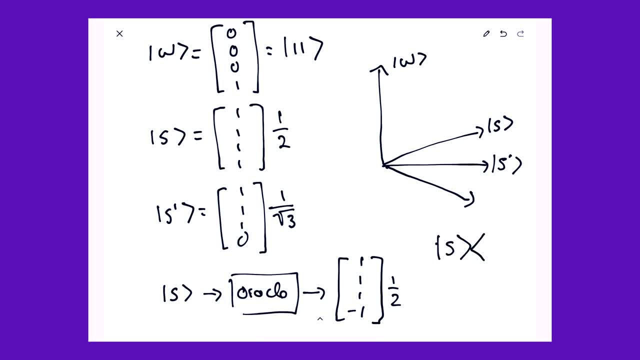 as the oracle. So we get a new vector that looks like this. So our S has been reflected around S minus the identity, And what this is going to do is reflect our new vector here about our original S vector. So what this looks like is something like this. So we started here, we went here. 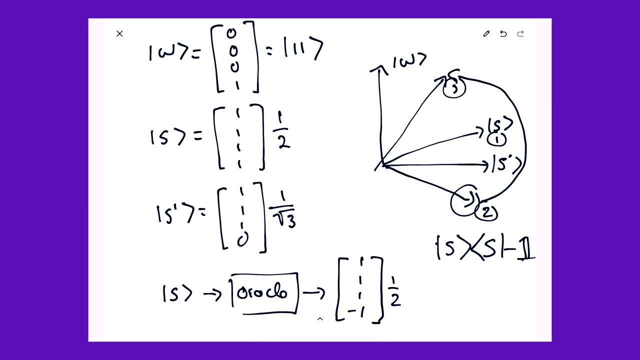 and then we ended up here. So you can see that the combination of these two operators actually brings us closer to our winning vector W here. In fact, each time we apply these two operators, our quantum state moves closer to the winning vector. In our example of four elements, 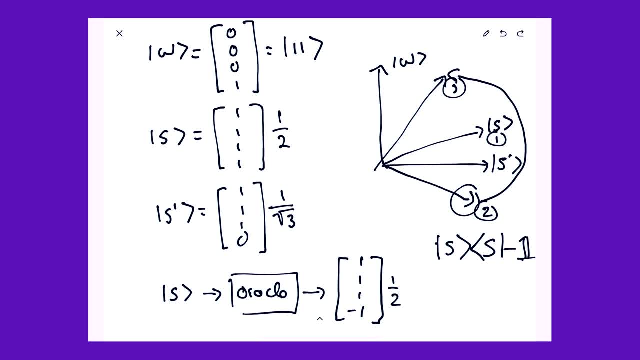 we'll see that we'll actually get the correct answer after one application of amplitude amplification For larger systems. the number of times we'll have to apply the amplitude amplification will scale as square root n. Let's take a look at how this works in Qiskit. We have all the pieces in place. 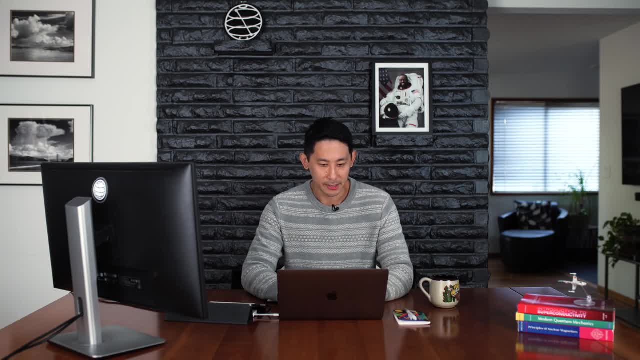 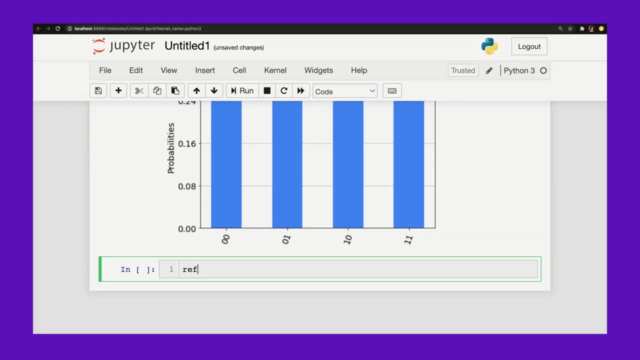 except for the reflection operator. now. So one way of thinking about the reflection operator is to apply a negative phase to every state orthogonal to our original S state. So let me start writing up this Action. So what we want to do is an operation that takes our superposition state back to the all-zero state. So we can do that. 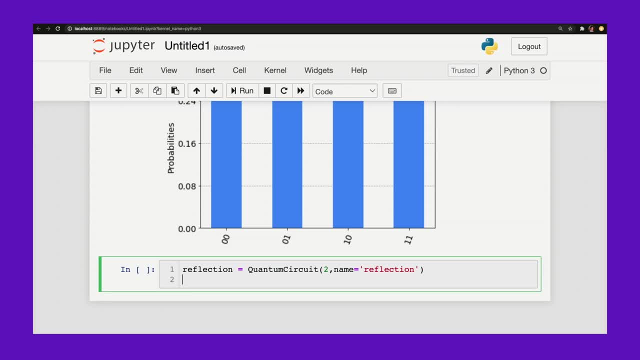 by applying Hadamards on every qubit And then apply a circuit that applies a negative phase only to the zero-zero state. So I'm going to add Hadamards on all of my qubits to bring them back to the original zero-zero state from the S state, And then I'll apply 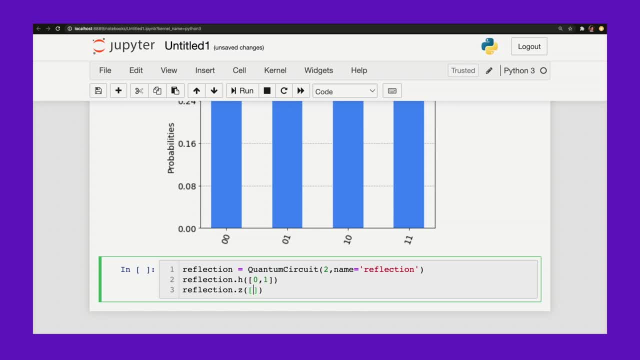 Z on both of my qubits and then a controlled C, And this is a circuit that will apply a negative phase only to the zero-zero state, And then I'll transform it back with the Hadamard on both qubits And I'll turn this on. 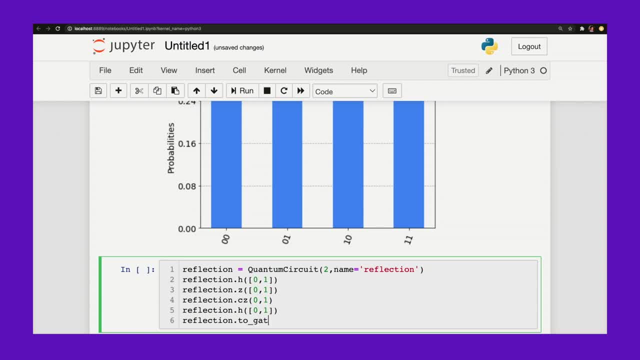 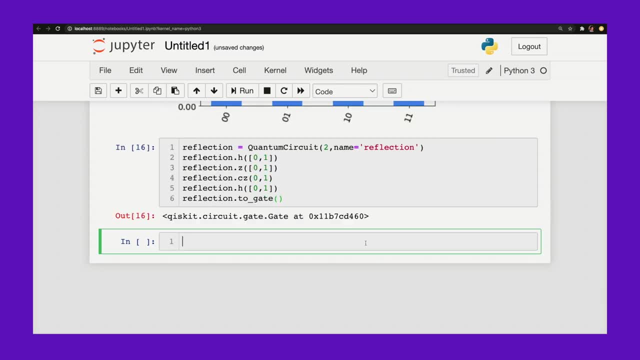 And see what happens. So there you go: pitch Ridge goes back to zero-zero state And then, yes, this also gives us a� grape, And then I'll donate this까 And I'll turn this into a gate. All right, and let's take a look at how the reflection operator looks. 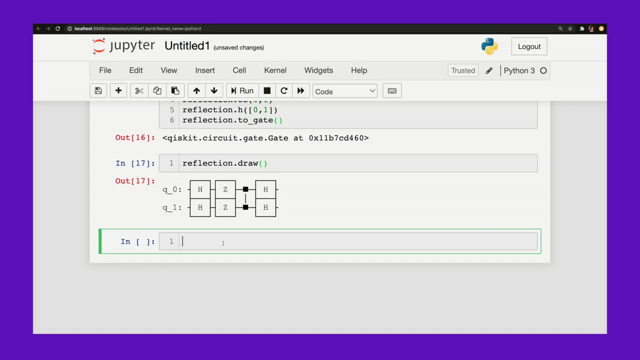 Okay, good, All right, and now let's put it all together. So I'll set my back end to the Chasm Simulator. Okay, overcirc equals quantum circuit, two qubits, two classical registers. I'm going to prepare my superposition state. 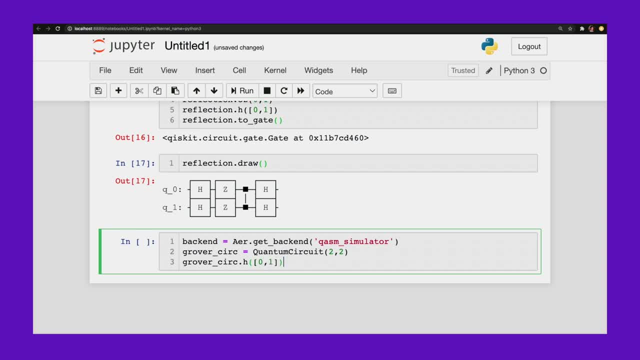 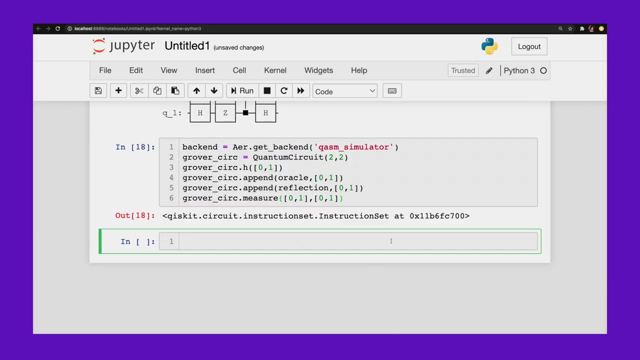 hadamards on both of my qubits, I'll add my oracle, And then I'll add my reflection operator, And then I'll add my measurements at the very end. Okay, and then let's take a look at what this circuit looks like. 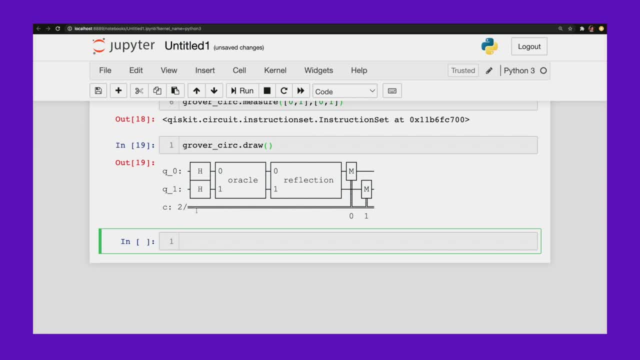 Okay, good. So we've prepared our superposition state, We have our oracle and we have our reflection operator, And what we want to get back at the very end is the state one one. So let's execute this job Overcirc. 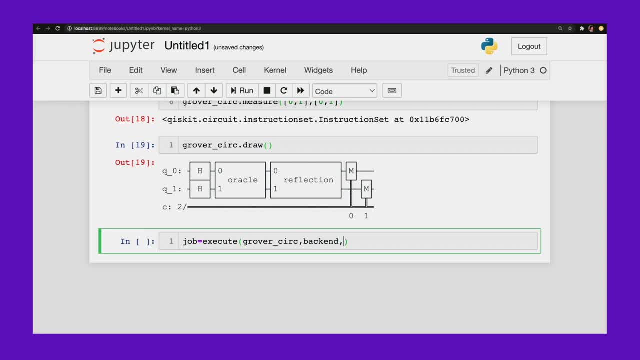 Back end And I promised you that we'll get the one one state back at the end. So I'm only going to do one shot. So let's get the result Result And get the counts back. Okay, great. So our result has given us back the one one state. 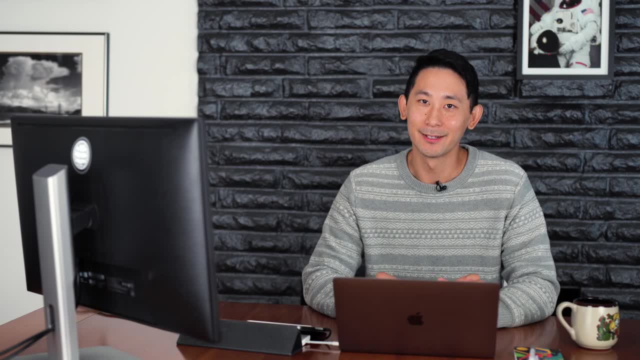 As promised. So there you have it. We implemented Grover's algorithm And we only use one call to the oracle in order to find our winning state. Now remember: classically we would typically need to use of order n calls to the oracle. 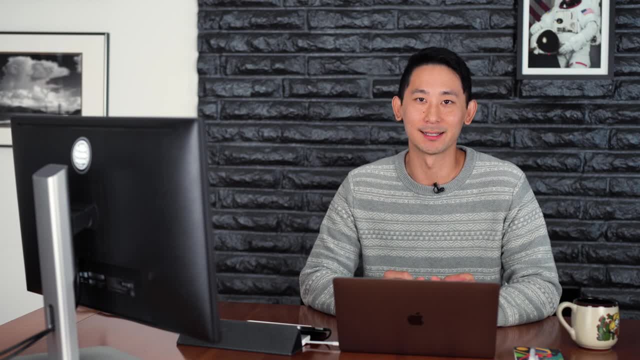 if we have an n size list. Well, in the quantum case, by using amplitude amplification, we can get away with only using square root of n. calls to the oracle. Why don't you try out this circuit on a real backend and let us know in the comments how? 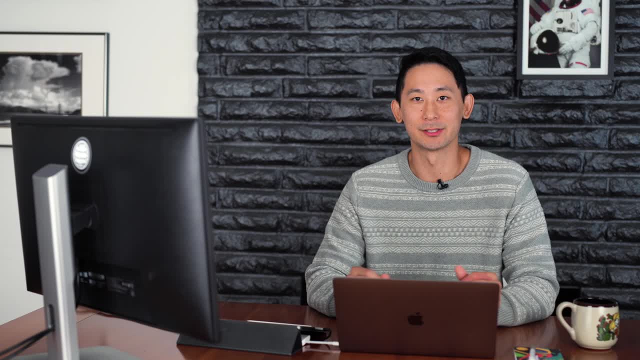 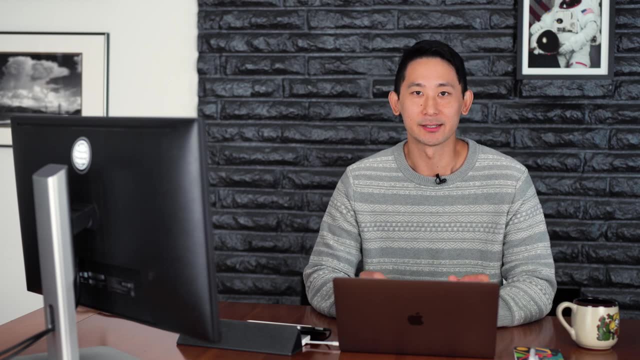